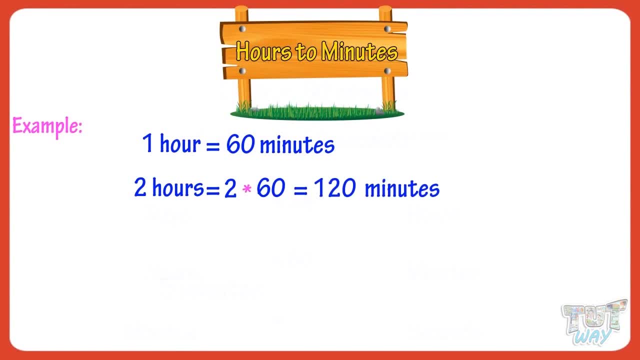 Multiplied by 60 equals 120 minutes. Now let's convert 3 hours into minutes. 1 hour equals 60 minutes, So 3 hours equals 3 multiplied by 60, that is 180 minutes. So, kids, for converting hours to minutes, you multiply the hours with 60. 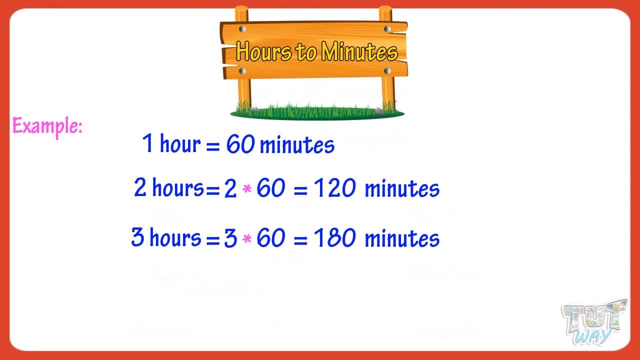 Now let's see more examples. 4 hours equals 4. multiplied by 60 equals 240 minutes. 5 hours equals 5. multiplied by 60 equals 300 minutes. Now let's convert 4 hours into minutes. Now let's learn converting minutes to seconds. 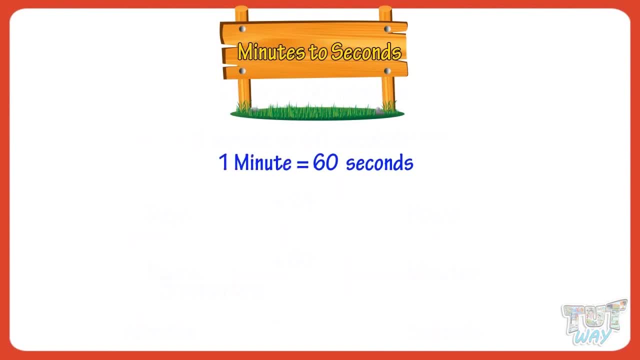 There are 60 seconds in a minute, So to convert minutes to seconds we need to multiply minutes with 60.. Let's see: 1 minute equals 60 seconds, 2 minutes equals 60 plus 60, or 60 multiplied by 2 equals 120 seconds. 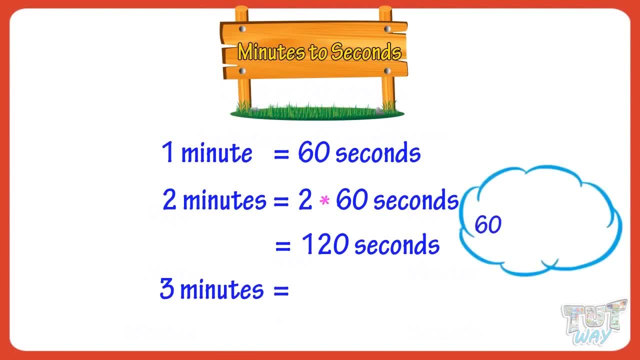 Let's see more examples: 3 minutes equals 60 plus 60 plus 60, or 60 multiplied by 3 equals 180 seconds. Now let's solve a few questions based on what we learned. It rained continuously for 2 days. 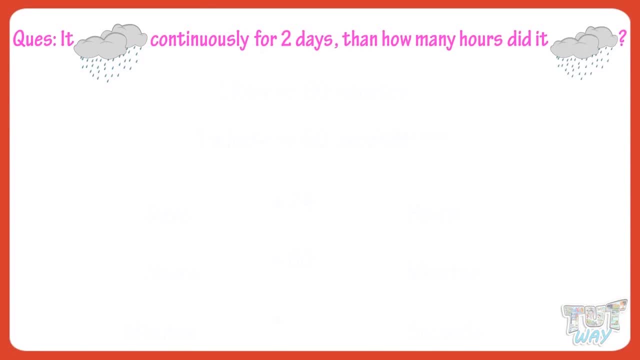 Then how many hours did it rain? 1 day equals 1 hour, 2 days equals 24 hours, 2 days equals 2, multiplied by 24 equals 48 hours. So it rained continuously for 48 hours. Now let's solve next question. 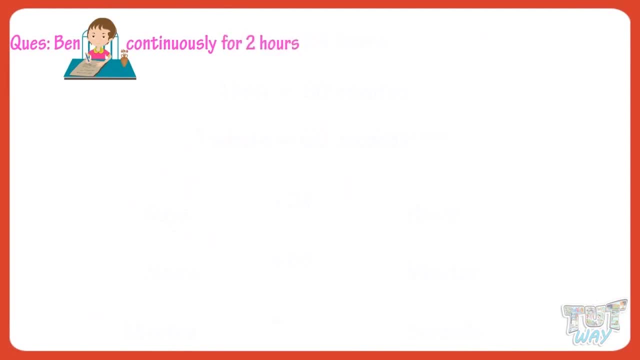 Ben wrote continuously for 2 hours. Then how many minutes did he wrote continuously. 1 hour equals 60 minutes. So 2 hours equals 60. multiplied by 2 equals 120 minutes. So Ben wrote continuously for 120 minutes. 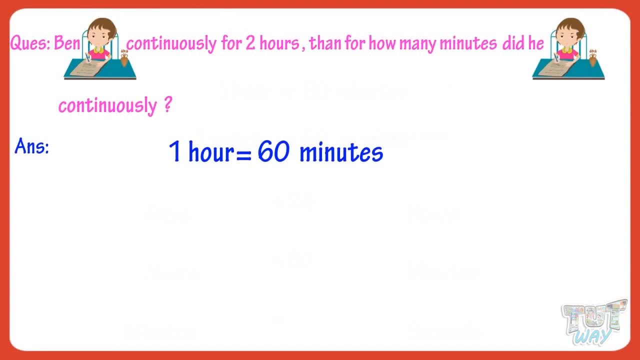 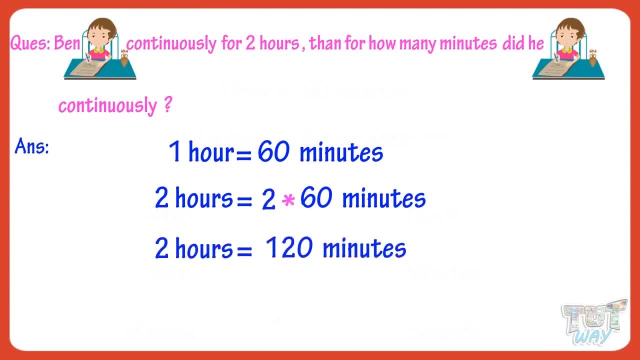 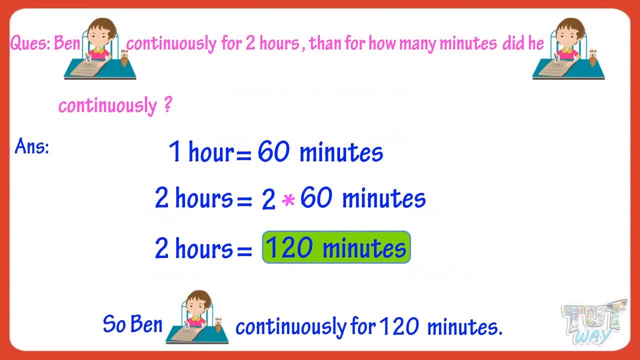 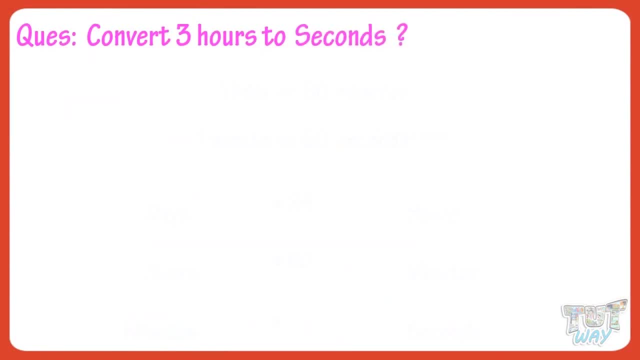 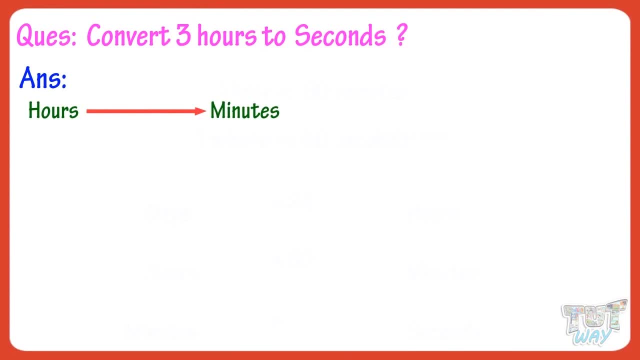 Let's first convert hours to minutes and then minutes to seconds. One hour equals 60 minutes, so 3 hours equals 60. multiplied by 3 equals 180 minutes. We have converted hours to minutes. Now let's convert minutes to seconds. 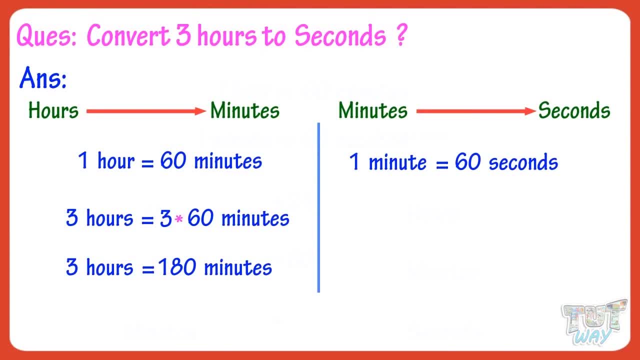 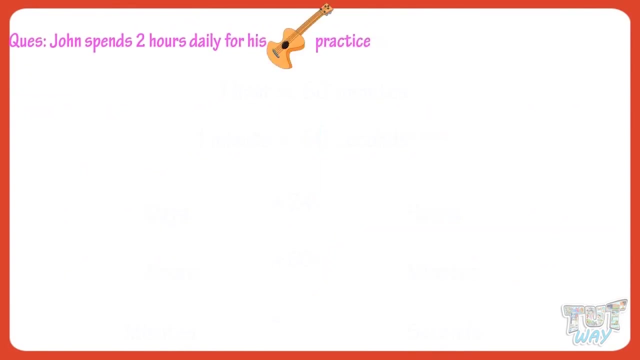 One minute equals 60 seconds, so 180 minutes equals 180 multiplied by 60 seconds, So it is 10,800 seconds. Now let's solve another question. John spends 2 hours daily for his guitar practice. If he practiced guitar for a week, then how many hours did he practice guitar? 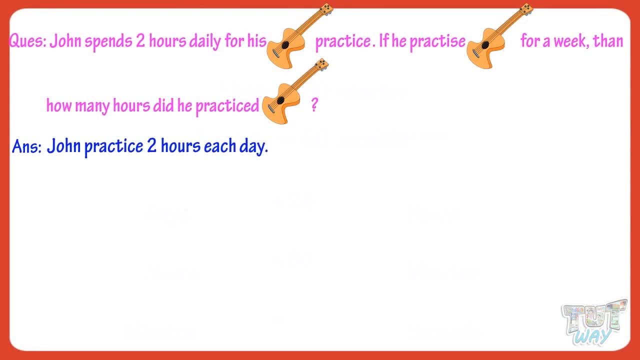 John practiced 2 hours each day. Number of days John practiced guitar: He practiced guitar for 7 days. as one week has 7 days, Number of hours he practiced in one day are 2 hours. So number of hours he practiced in 7 days will be 7 multiplied by 2.. 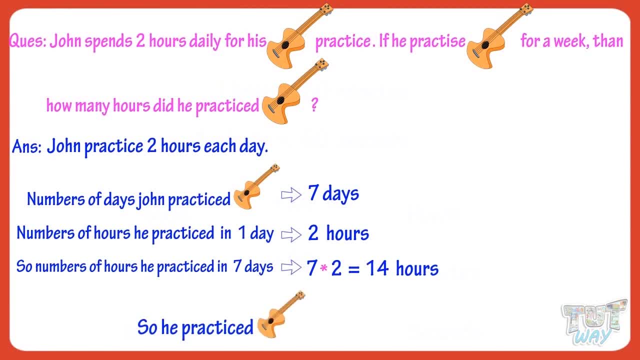 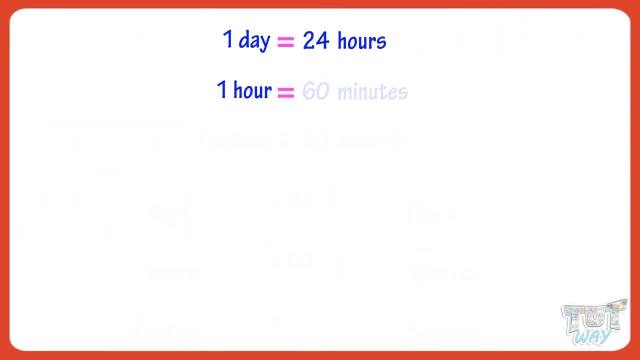 That is 14 hours. So he practiced guitar for 14 hours in total. So, kids, today we learned that One day equals 24 hours, One hour equals 60 minutes, One minute equals 60 seconds And to convert days to hours, we multiply.